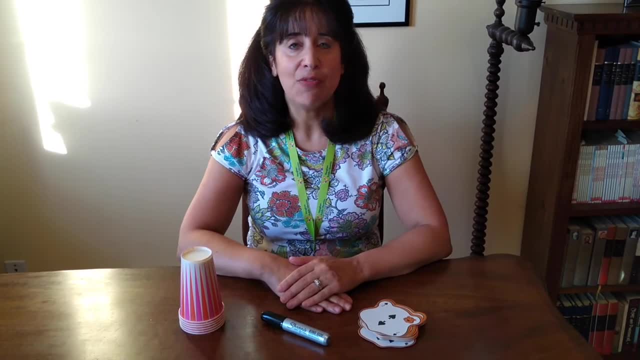 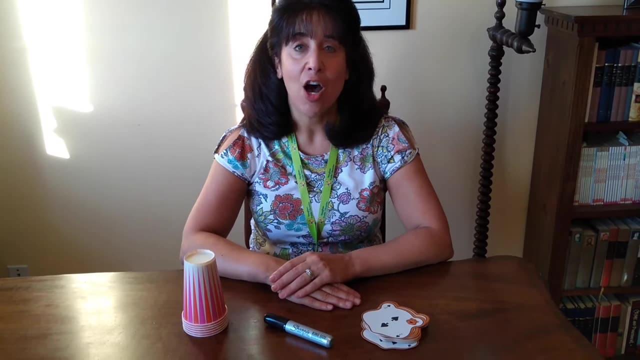 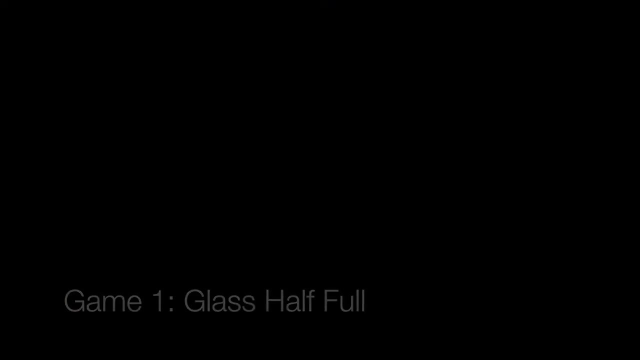 Simon says Geometry is number three, and this is a review of geometry vocabulary. using only one's arms, The only supplies are some plastic cups, a Sharpie and a deck of cards. The game is a little bit more complicated, but it's worth it. Let's get started. 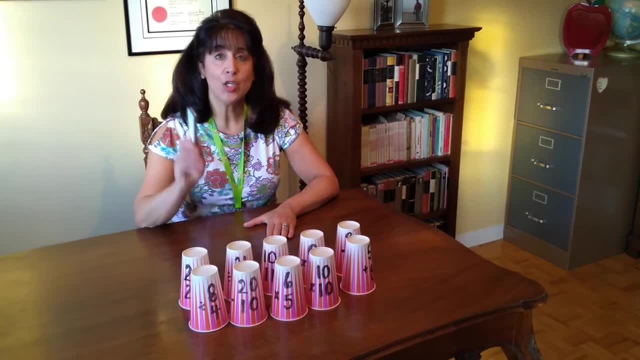 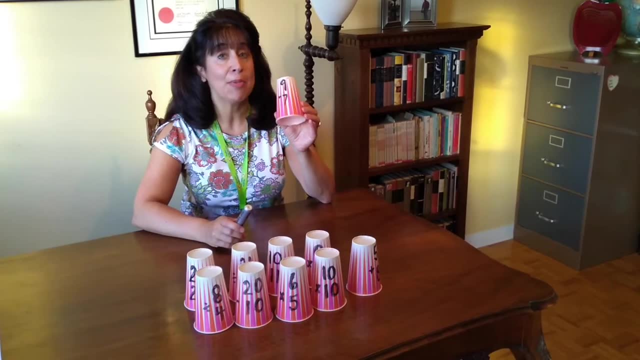 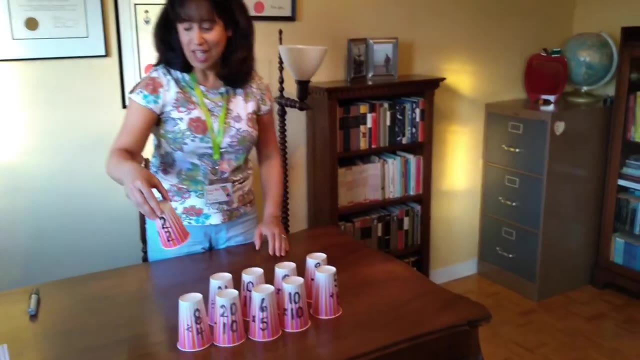 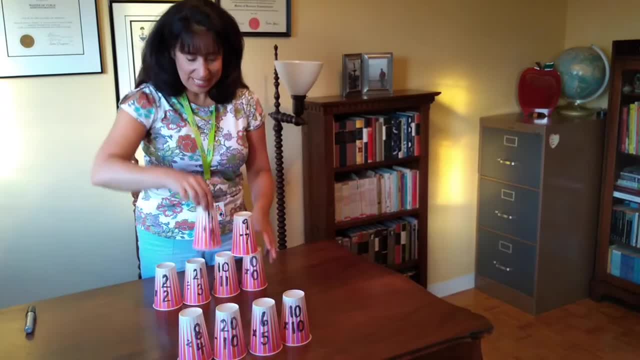 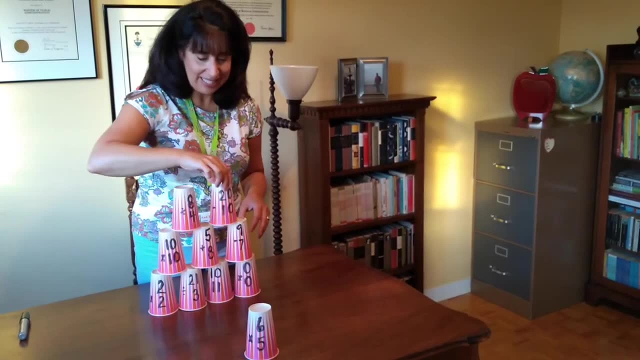 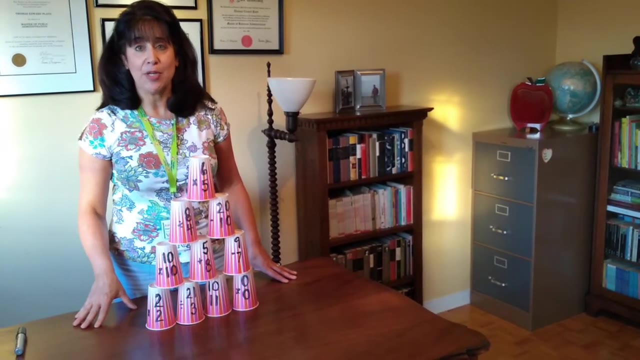 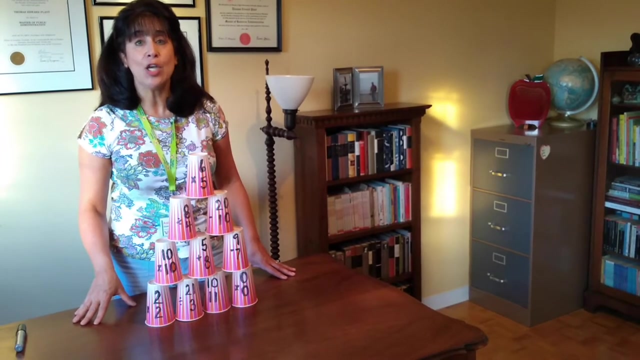 Two Thirteen, One hundred Two Ten Thirty. To change it up, involve a time component or include another child with their own set of stacking cups and make it a little bit more competitive by seeing who can stack all of their cups first. 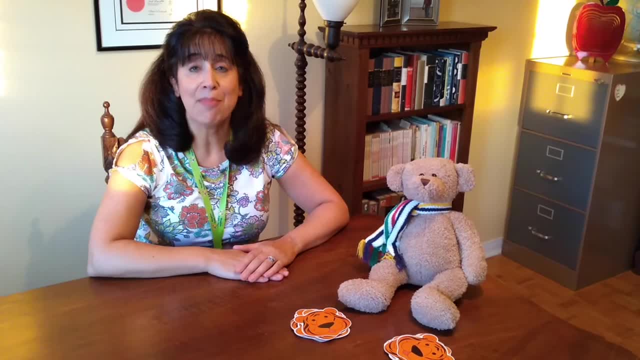 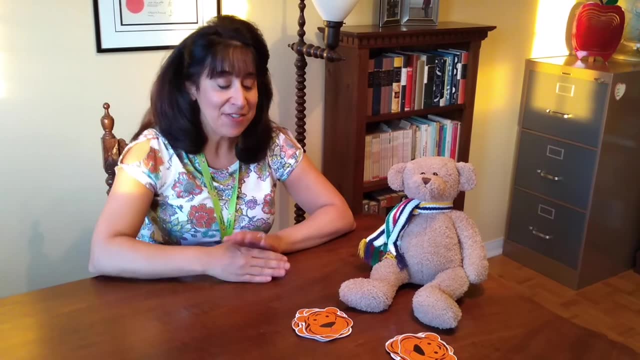 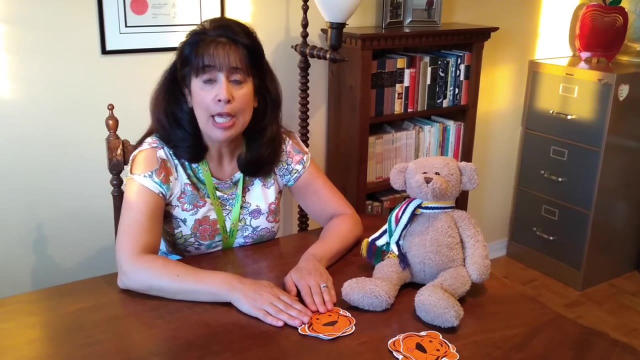 For this game, a minimum of two players is needed. Teddy will help you demonstrate. Sounds like fun. Divide the deck equally. Please note that I have removed the Ace Jack, Pink and Queen, but you can leave them in, just to assign a number value for each. 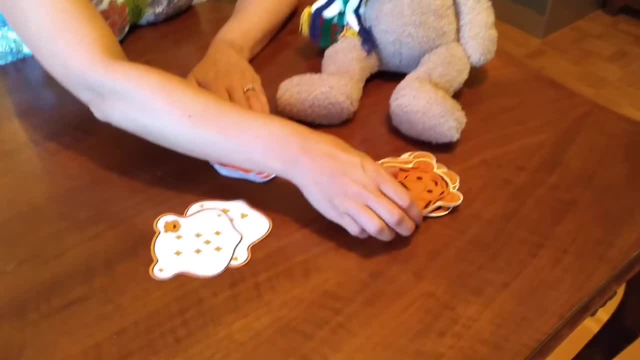 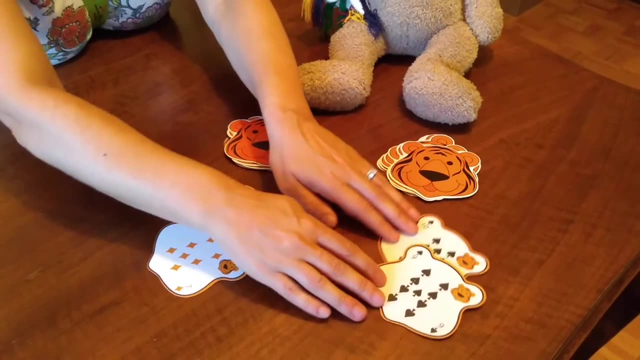 Each player flips two cards at a time. I'll flip yours, Teddy. Thanks. The highest sum gets all of the cards. So if we look at Teddy's, you have a 10 and a 9.. So what is 10 plus 9?? 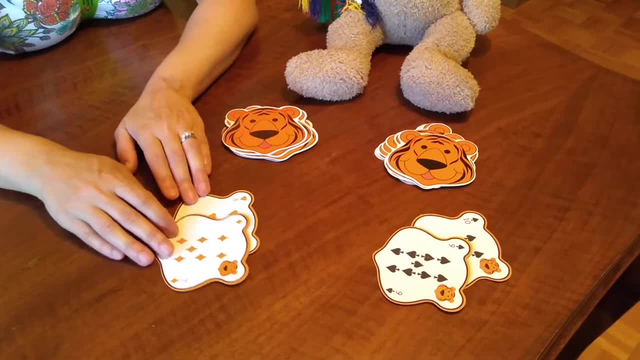 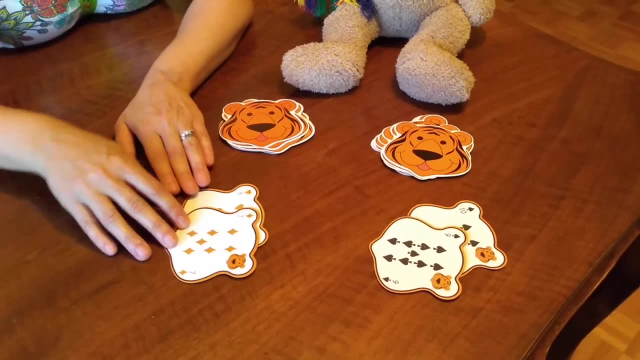 15.. That's right, And I flipped an 8 and a 7, so that makes 15.. So, Teddy, 19 is higher than 15, so you get all of the cards for this round. Hooray, And so forth.